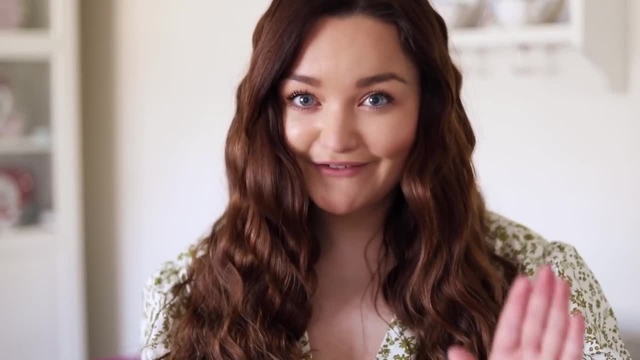 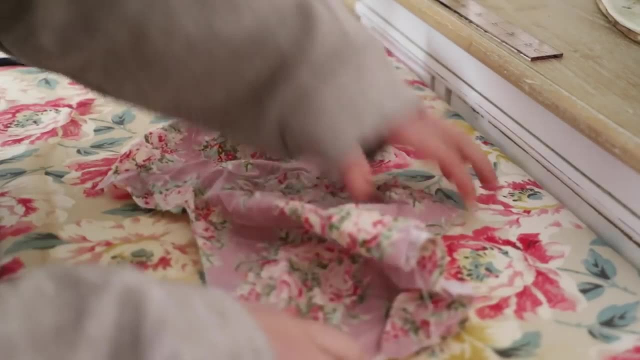 half an hour if you are a pro. But these are scrap fabric. friendly, Hands up who has balls of fabric creased, stuffed into a bag and they're like, hmm, I don't want to throw that out, but I can make something with that. I'm gonna pop timestamps below and I've tried to put all of the measurements. 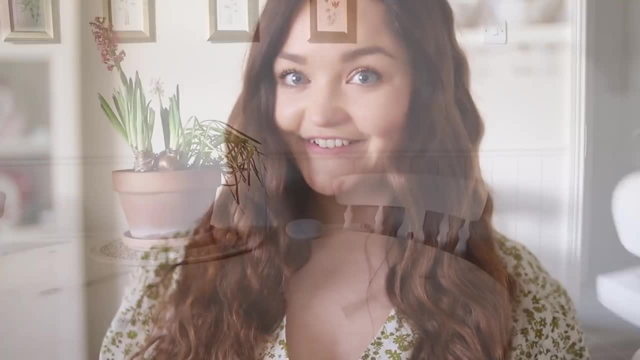 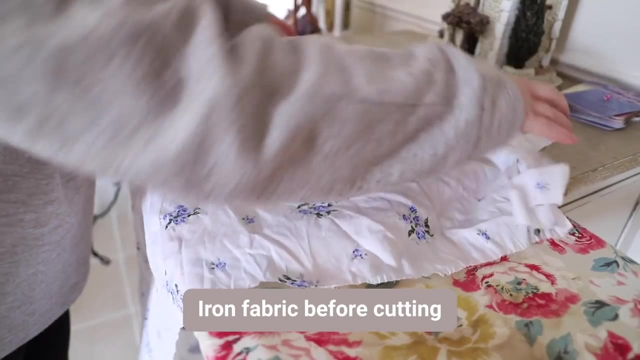 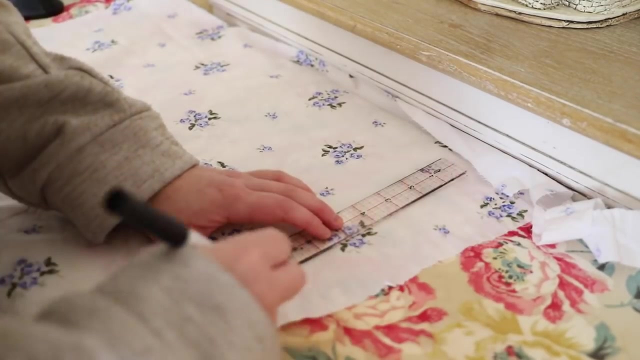 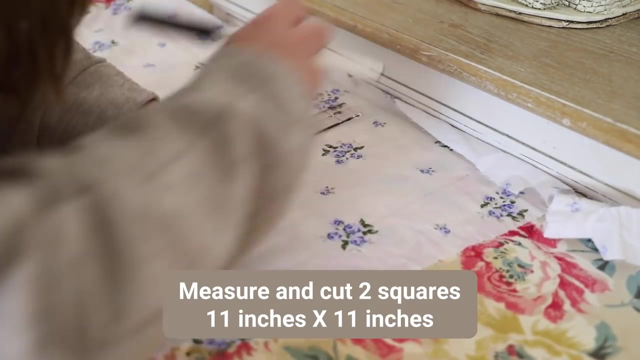 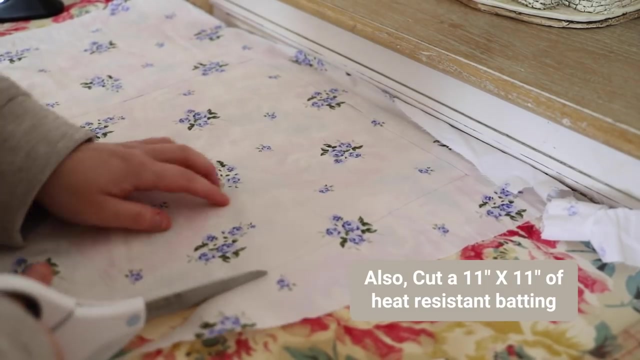 on screen as well, but I'll pop them in the description for you also. Please give me a thumbs up, and if you have any questions that I might answer, I can answer them in here. so please do so. I will see you in the next episode. bye. 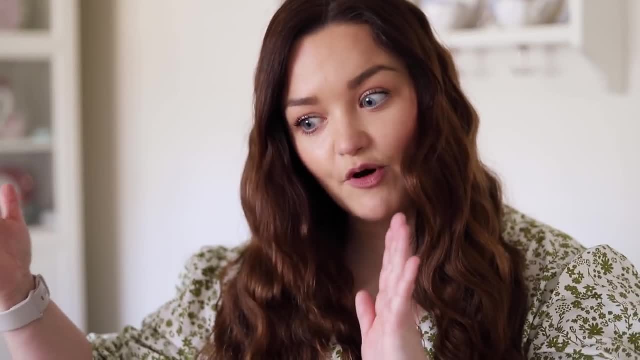 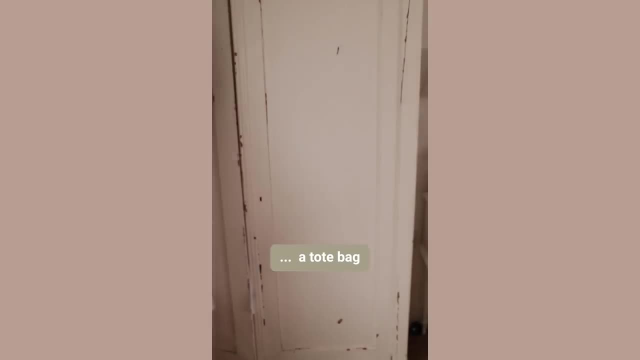 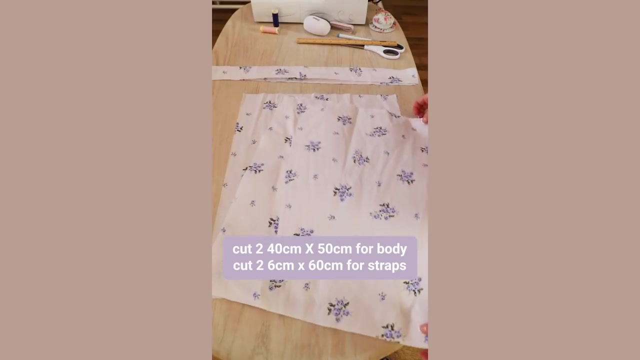 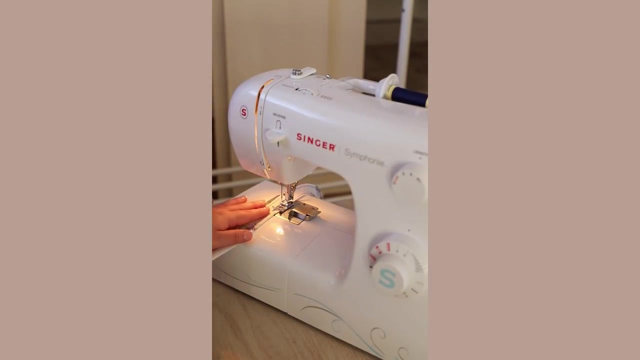 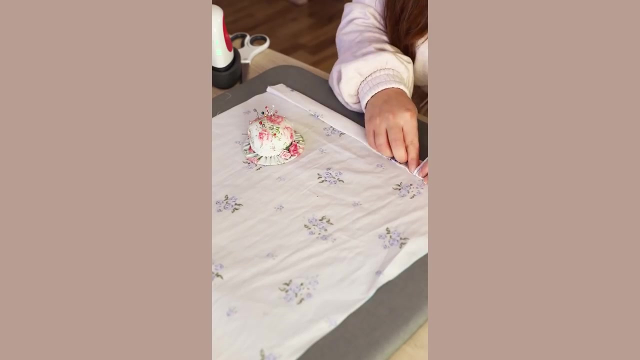 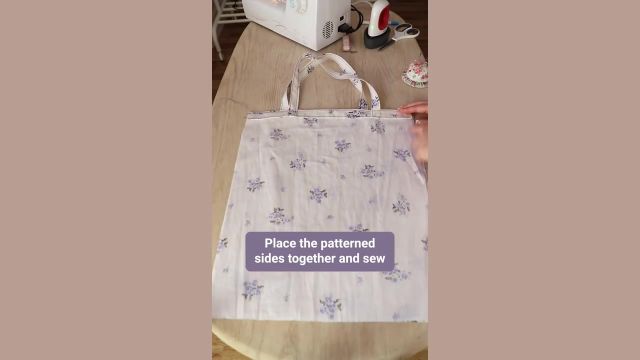 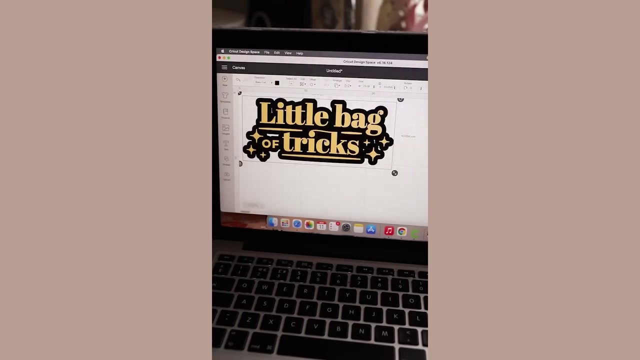 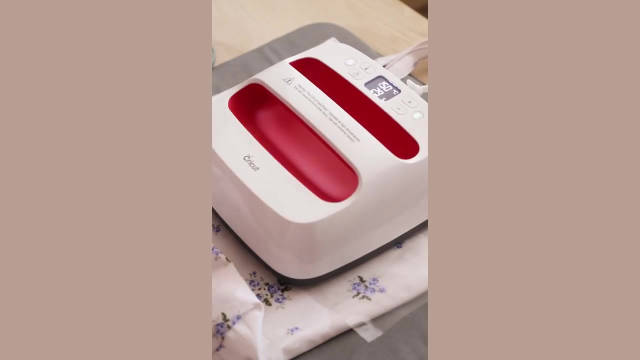 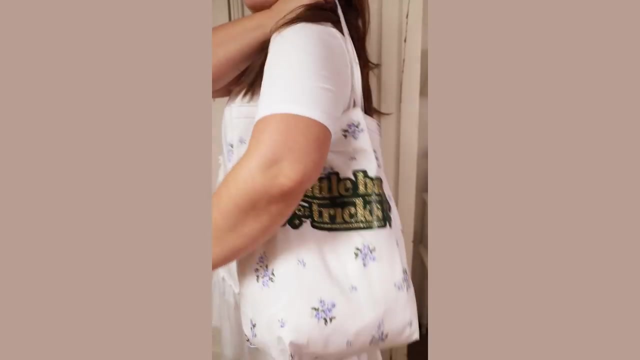 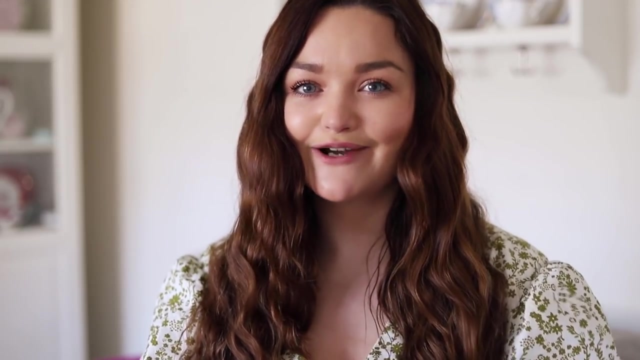 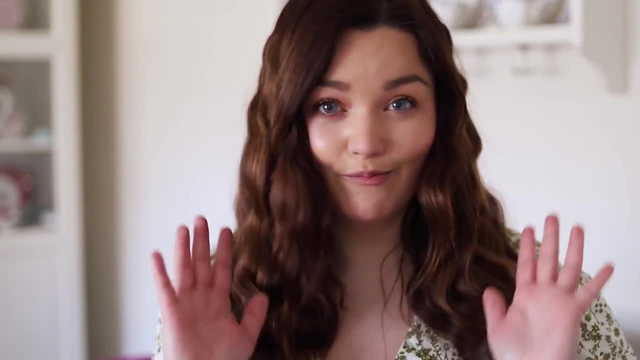 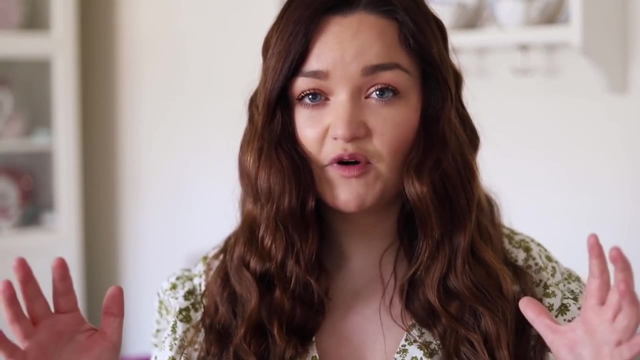 of just sit and sew, but I do have more sewing projects, So I have a video and I'm going to pop a card in here and that video. I think there's 10 sewing projects and, again, beginner friendly, you can do them in under an hour. scrap fabric. 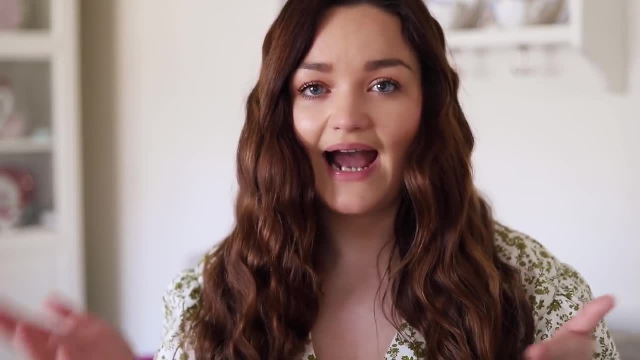 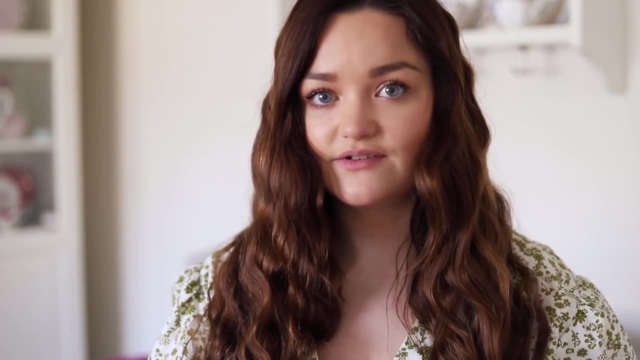 friendly. but I think take the idea and make them. There's not enough money, them your own if you want to add bits of fabric, if you want to like do patchwork or something you could totally like, experiment and just take the measurements and just tweak them. take the idea. 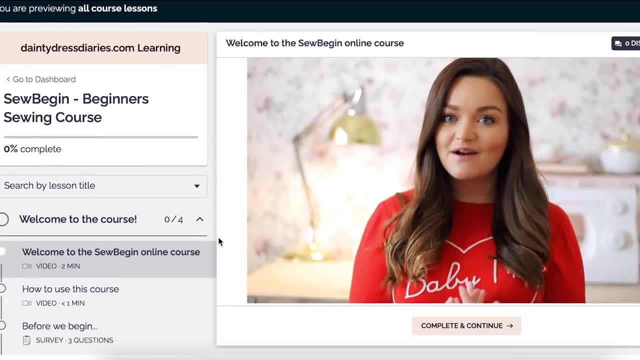 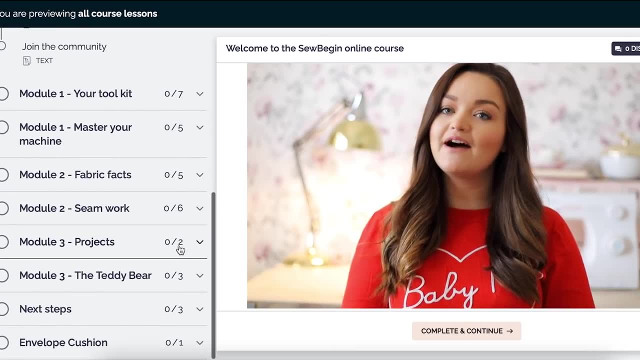 and make it your own. also, if you are an absolute beginner but you want to get started and you're like: i don't even know how to thread my machine, i have an online beginner sewing course that is geared towards beginners who, if you don't know how to thread your machine, it will take you through. 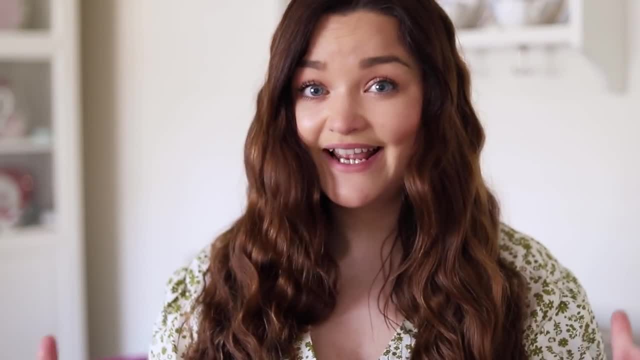 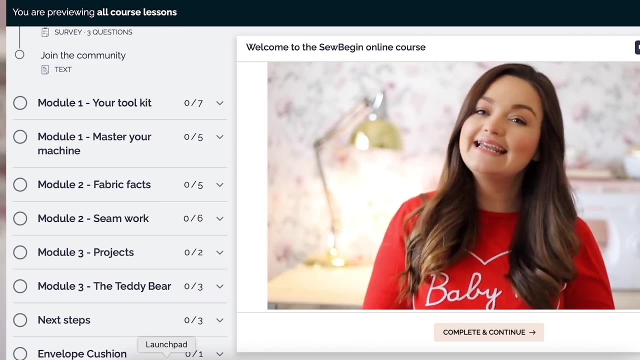 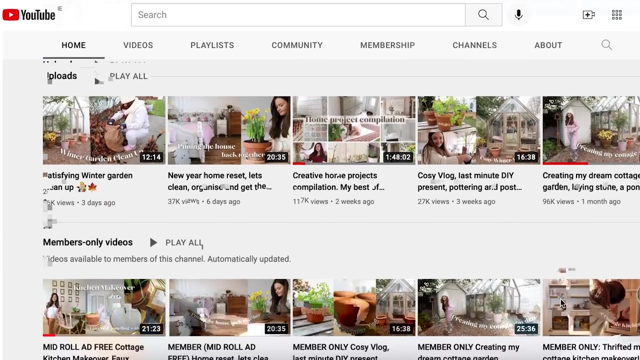 all of the basics, because if you can master the basics then you can go on and tackle more advanced projects. i'm going to pop a link with more info on my sewing course in the description. also, youtube members get a mahoos of discount on the sewing course. so if you want to find out more info, if 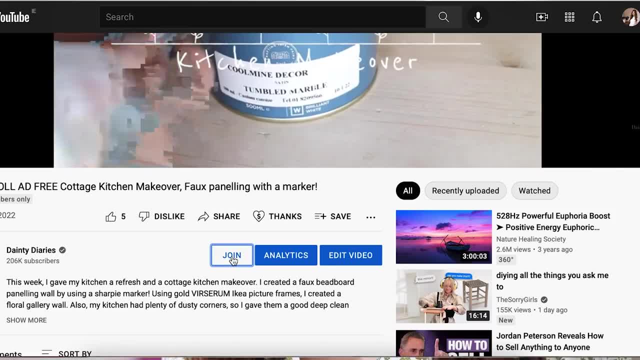 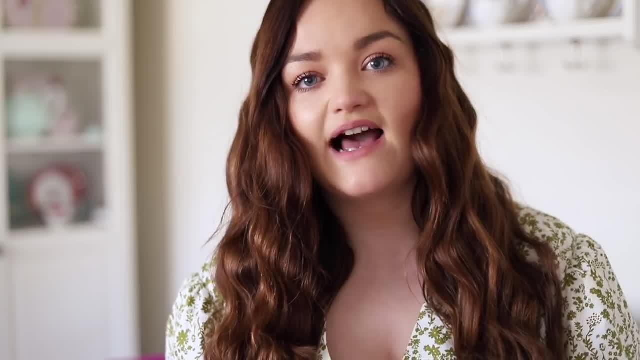 you hit the join button underneath, i think me and it'll give you more information on what you get with a channel membership. so i upload my weekly videos earlier for members and mid-roll ads are removed so you can get more information on what you get with a channel membership. so i upload my